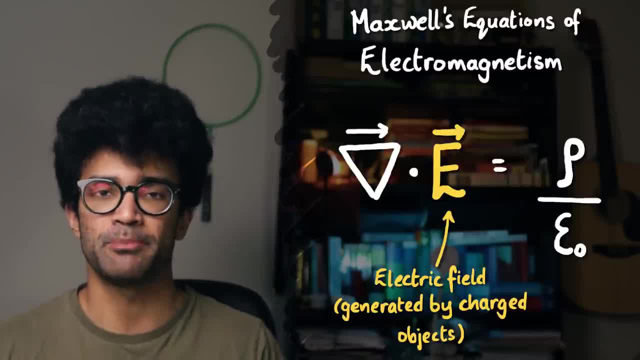 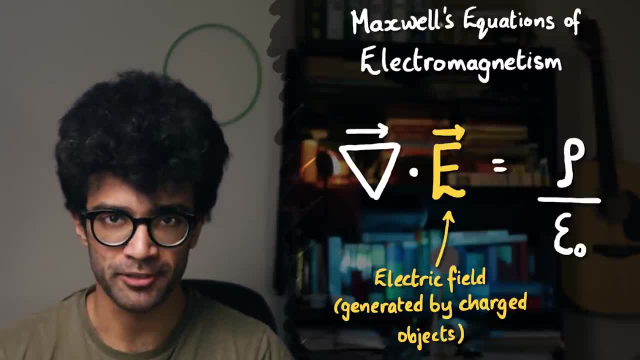 of electric fields. These electric fields are generated by charged particles or charged surfaces or charged objects in general. We'll look in a bit more detail in a moment what we mean by electric fields, but let me start out by saying that an electric field is a very specific. 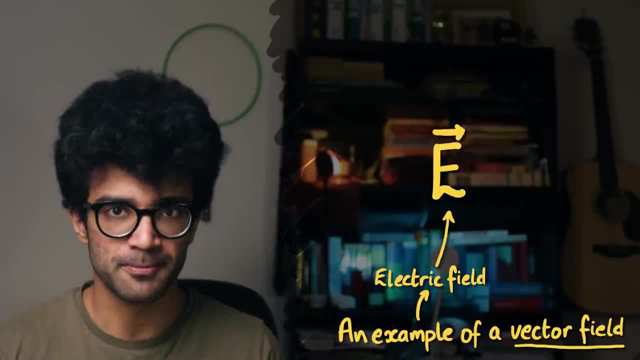 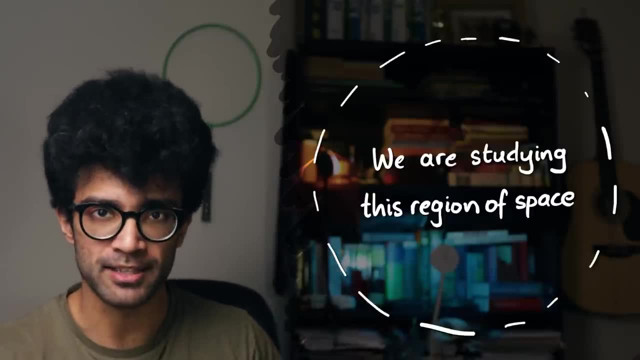 kind of example of something known as a vector field, basically a field of vectors. Let's say, for whatever reason we happen to be studying this region of space and we're studying a vector field in that region of space, Well, we can think of a vector field as basically this region of space. 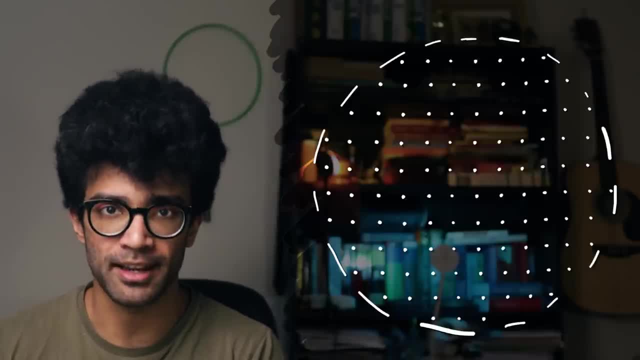 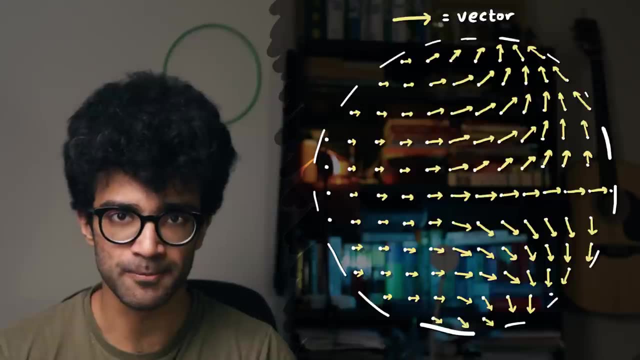 and every single point in that region of space can be assigned a particular vector Vectors, of course, being represented by an arrow with a certain length and pointing in a certain direction. We're not talking about electric fields specifically, just yet. We're just thinking of a general vector field. In a general vector field, these vectors 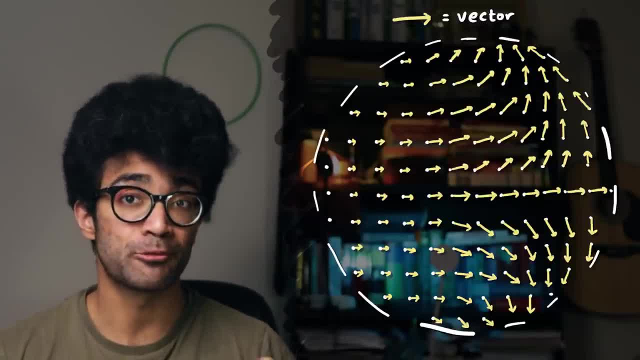 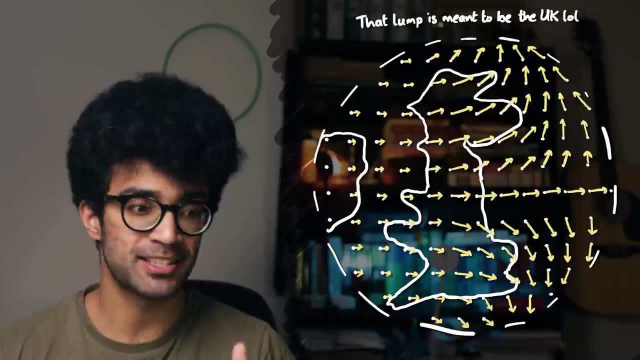 can represent one of many things. For example, this could be a vector field representing the speed and direction of wind at each point above the United Kingdom. Or we could have a vector field that describes the direction and speed of little sneeze particles that come out every time. 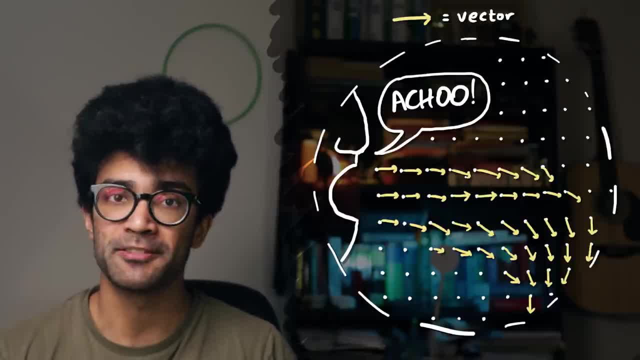 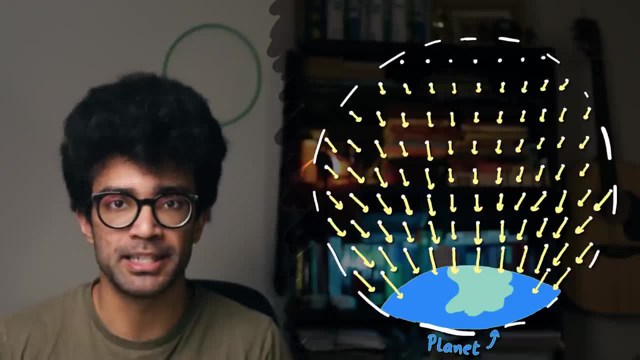 somebody sneezes Topical right. Or we could have a vector field that describes the size and direction of the gravitational force exerted by a planet on a mass placed at a particular point in that vector field. If you want a more in-depth discussion of vector fields, then I've talked about these in my first. 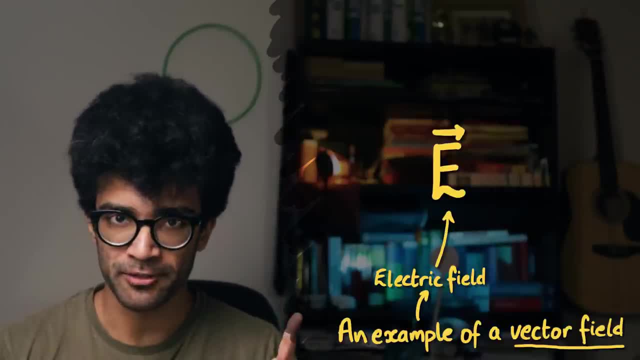 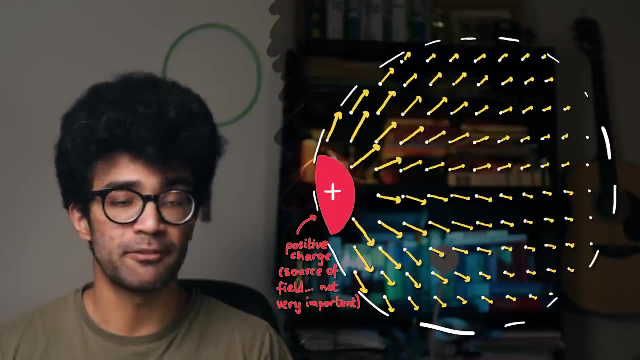 Maxwell equation video. Check it out up here. But now let's look at electric fields. Electric fields being a particular example of a vector field, Here is an electric field. This field represents something very closely related to the force exerted on a charged particle. 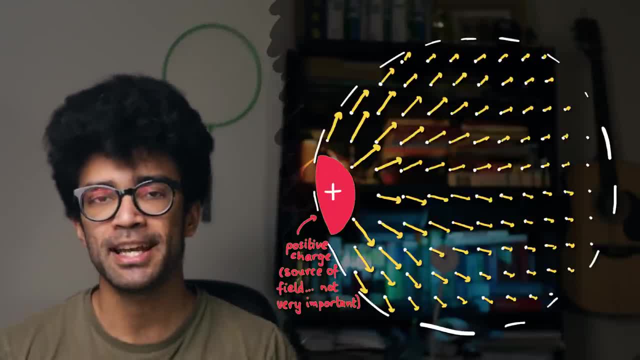 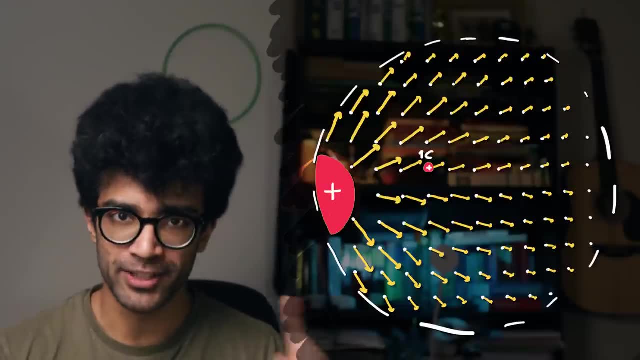 that we place at any point in that field. Basically, if we take, let's say, a positively charged particle and this charged particle we can say has a charge of one coulomb and we place it at this particular point in the electric field, then this diagram tells us that this one coulomb 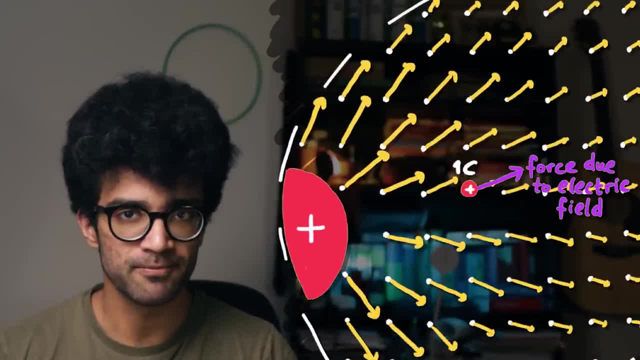 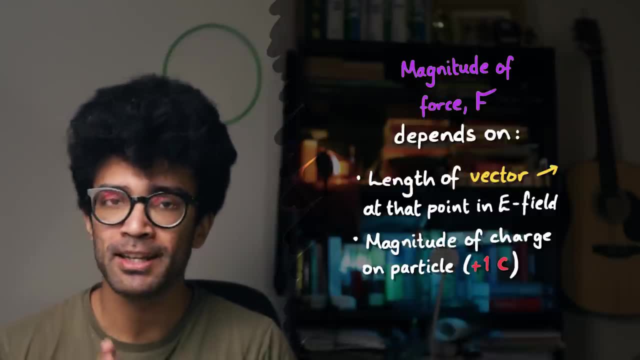 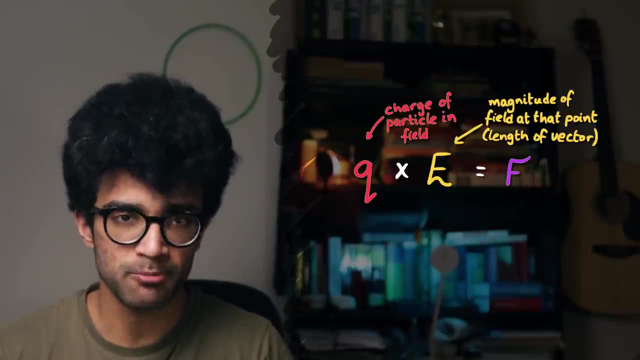 charged particle would experience a force in this direction. The magnitude or size of that particular force is directly related to both the size of the vector starting at that point as well as the magnitude or size of the charge, Specifically the length of the particle multiplied by the length of the vector or the size of the arrow. 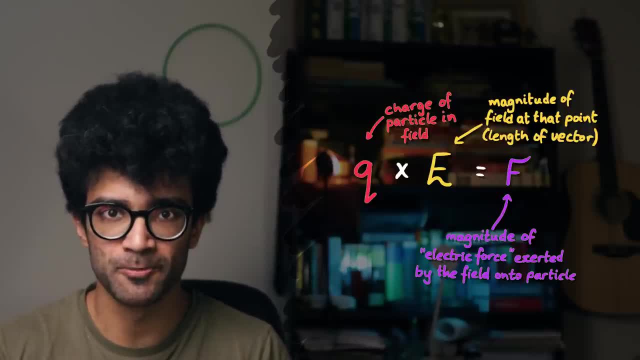 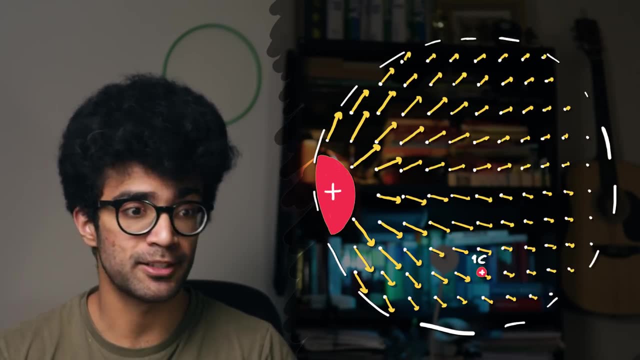 gives us the magnitude or size of the force exerted on that charged particle. As a clarifying example, we could take that same charged particle and place it now here in the field. This diagram tells us that the force exerted on our charged particle when placed here. 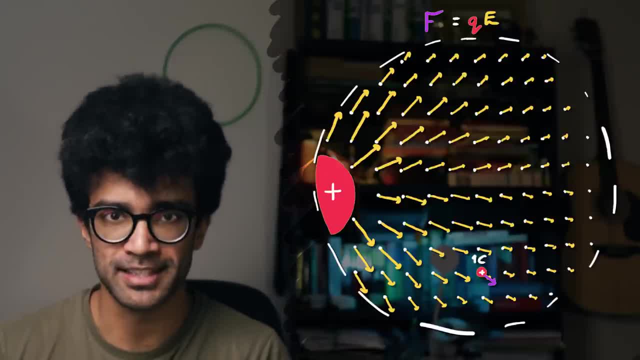 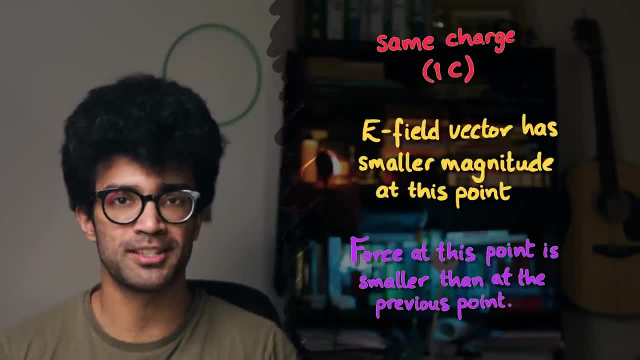 will be in this direction and will have a smaller magnitude. in this case, because, even though the charge on the charged particle is still one coulomb, the original vector had a smaller magnitude and so the force exerted on the one coulomb. 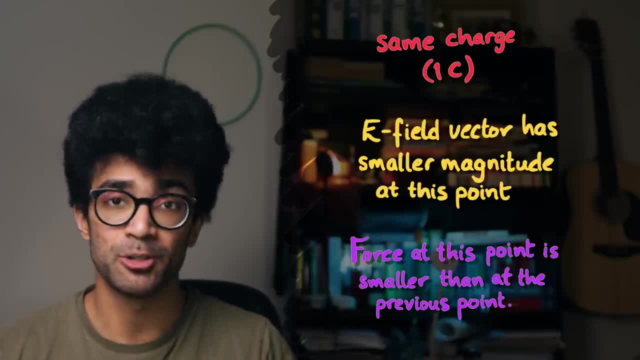 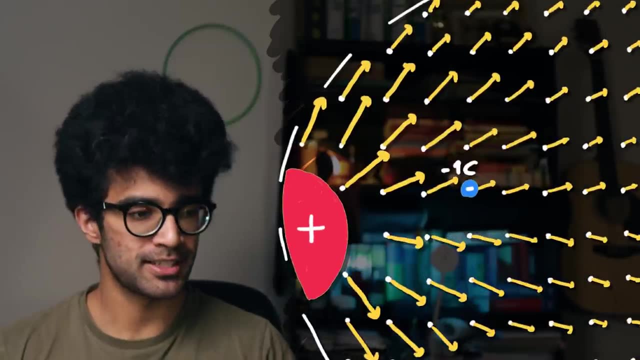 charge is going to be smaller at this location. And just to clarify things a little bit more, if we took a negative one coulomb charge and placed it in this electric field, let's say at this point once again, then the force exerted on this 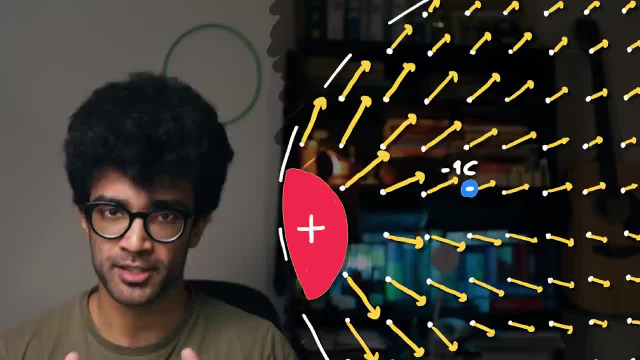 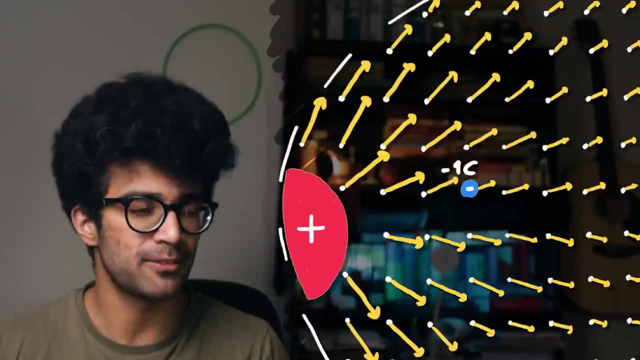 negatively charged particle would be equal to the magnitude or size of the vector multiplied by the charge. but this time the charge is negative. So the force exerted on our negatively charged particle is going to be in the opposite direction to the force exerted on the positive particle. 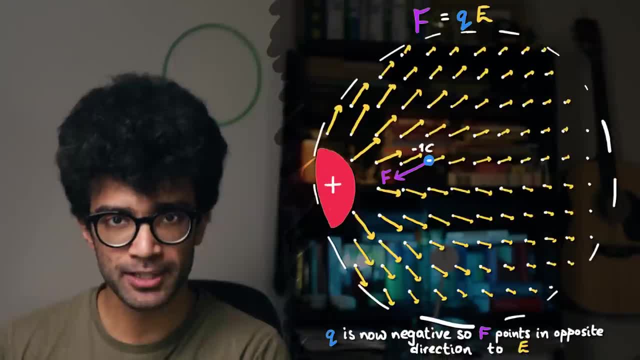 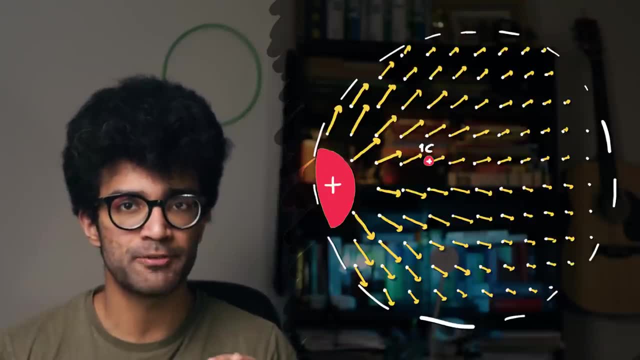 because both the positive and the negative charges we considered have the same magnitude. the forces will be of the same magnitude, just in opposite directions. So this teaches us something important: When we take a positive charge and place it in an electric field, the electric field diagrams are drawn in a very specific way, such that the force 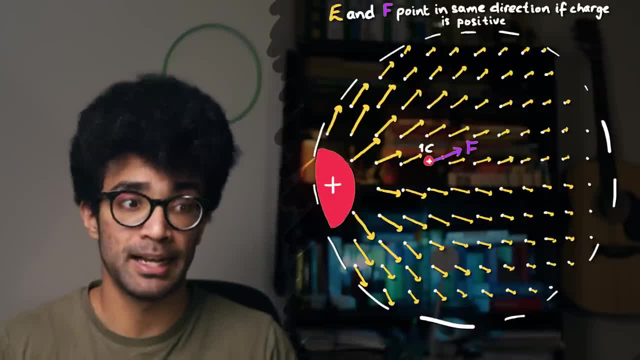 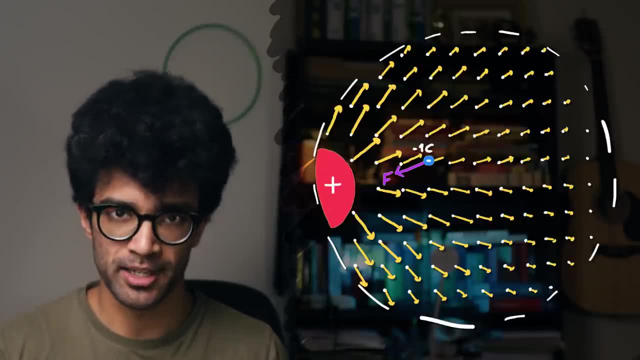 experienced by a positive particle is in the same direction as the electric field diagram, and the force experienced by a negatively charged particle is in the opposite direction to the arrows or the vectors drawn in our diagram. This is by convention. Scientists sat down a long time ago and decided that the vectors used to 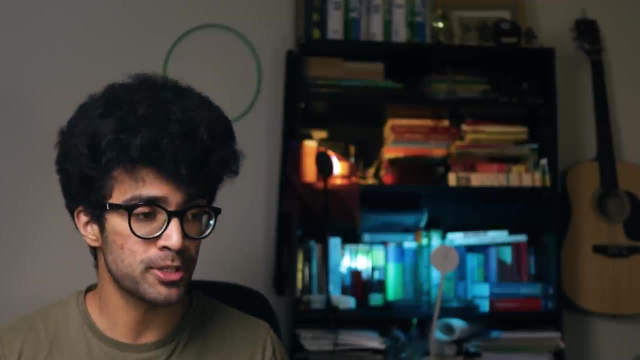 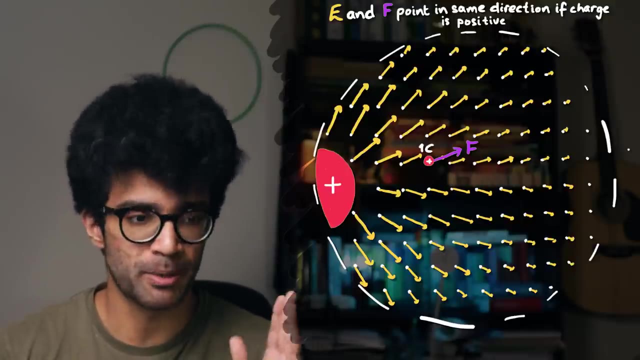 represent electric fields will be pointing in the direction of forces experienced by positively charged particles. It's just a choice, basically It doesn't really matter. but the majority of the physics world goes by this convention. But, more interestingly, we also learn that the force 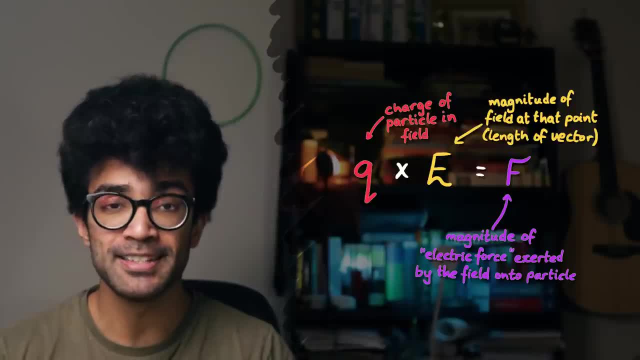 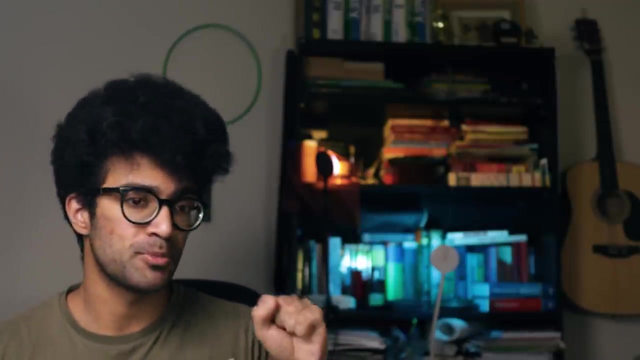 experienced by a particular particle in an electric field is equal to the charge on that particle multiplied by the magnitude of the vector at that particular point in the electric field. So the electric field is a representation of forces felt by charged particles, whilst also removing the dependence on the charges of those charged particles. So, coming back to our equation, 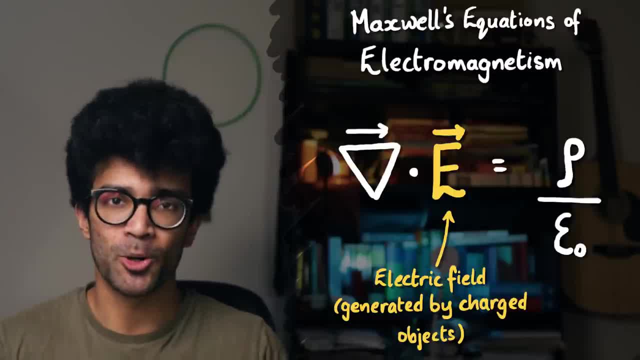 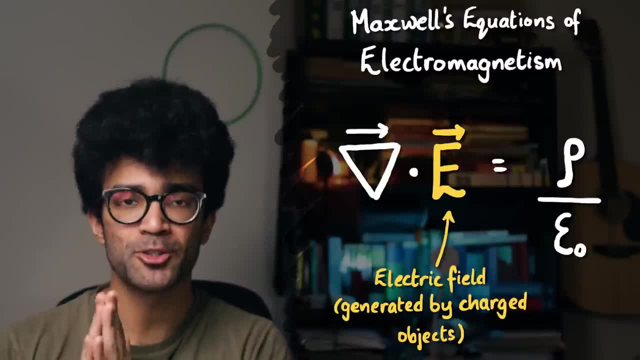 from earlier. that's what the E stands for. The E represents the whole of the electric field And you'll notice that there's an arrow above the E. This tells us that it's a vector or vector field. But anyway, that's not so important. Next, what we can do is to look at what this downward pointing. 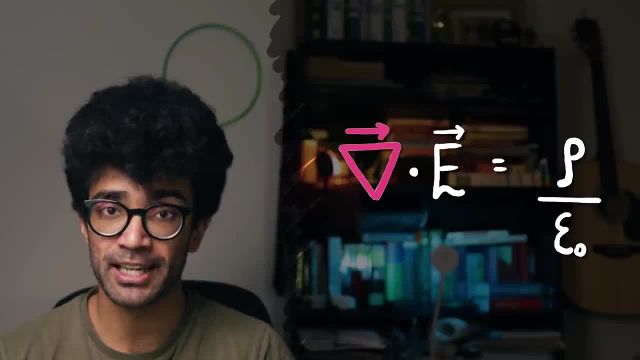 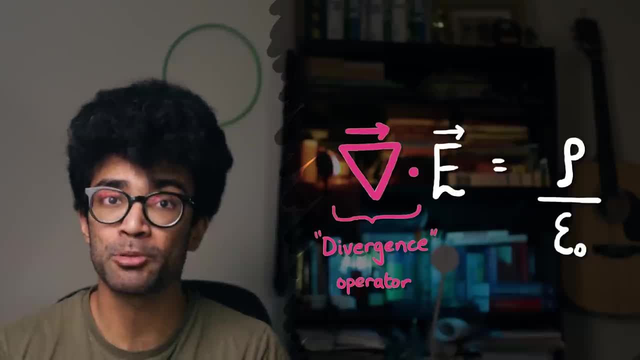 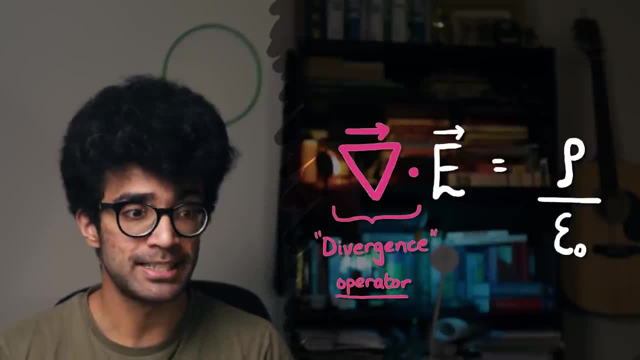 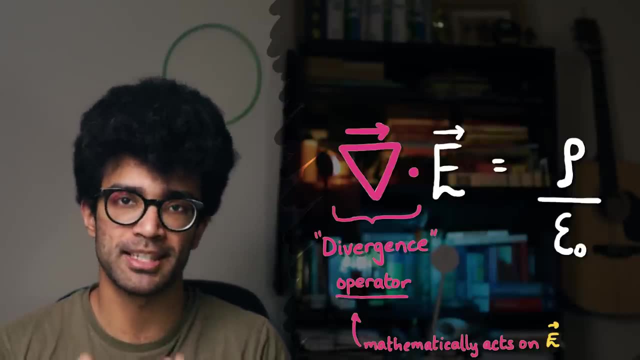 what that means. First of all, like I said, we're dealing with an operator, It does something mathematically to our electric field representation. And secondly, this particular mathematical operator is known as the divergence operator. And so, just out of interest, if we want to read, 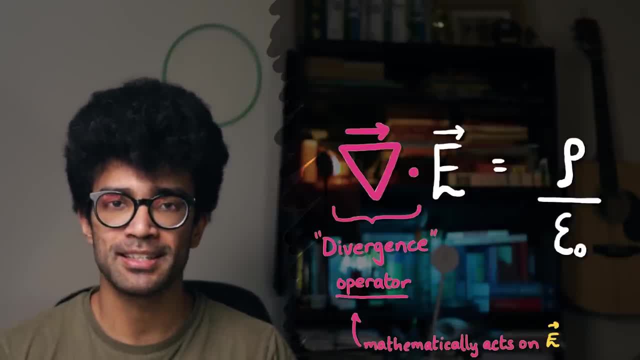 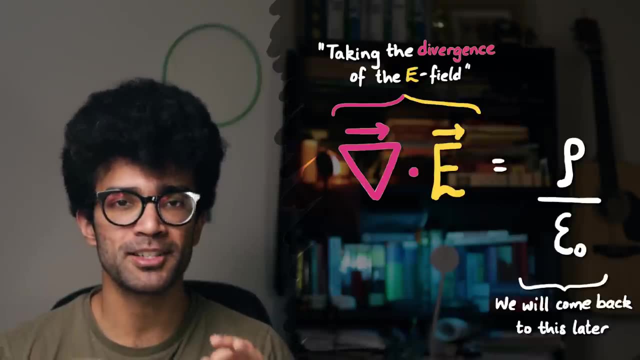 or interpret the left-hand side of this equation. we can say that this is taking the divergence of the electric field E. We'll come back to the right-hand side of this equation in a moment, but first let's look in a bit more detail at the divergence mathematical operator. 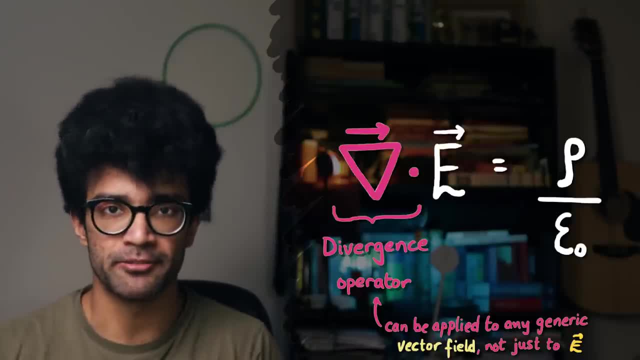 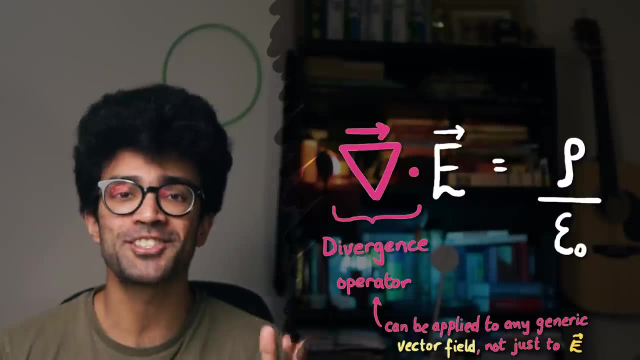 Again, this divergence operator can be applied to any generic vector field, not just, specifically, the electric field. But what do we mean by finding the divergence of a vector field? Well, to answer this question, I am bringing out the big guns, That's right. Mr Higzino is going to be answering. 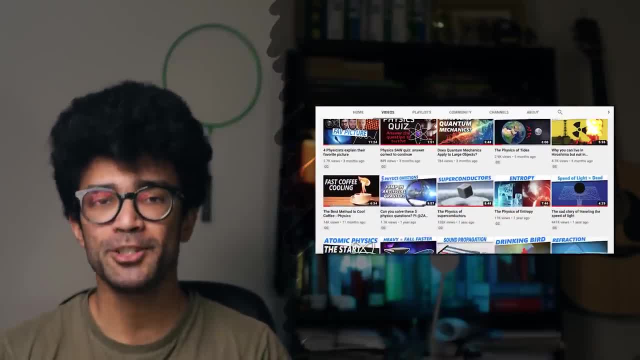 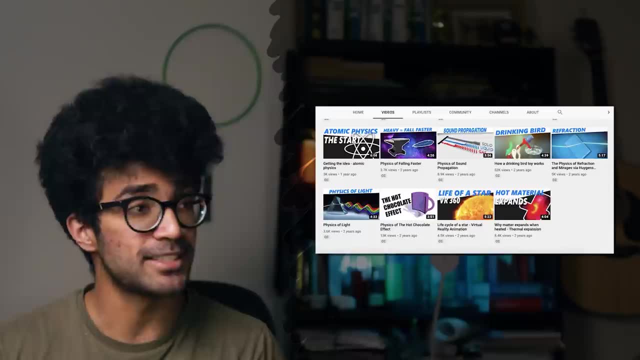 this question for us. He's going to show us a very intuitive and visual way of understanding what it means to take the divergence of a vector field as opposed to just a mathematical understanding. Take a look. Thank you very much for inviting me, Paul Talking about one of the best equations. 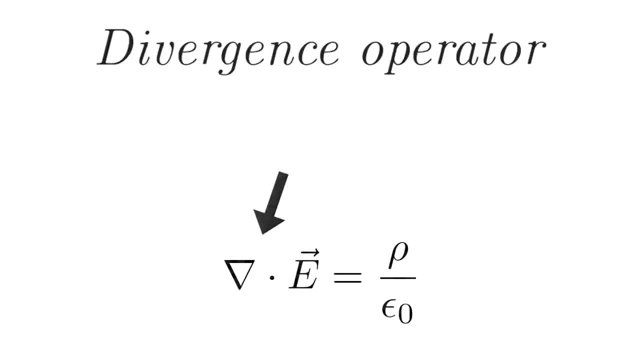 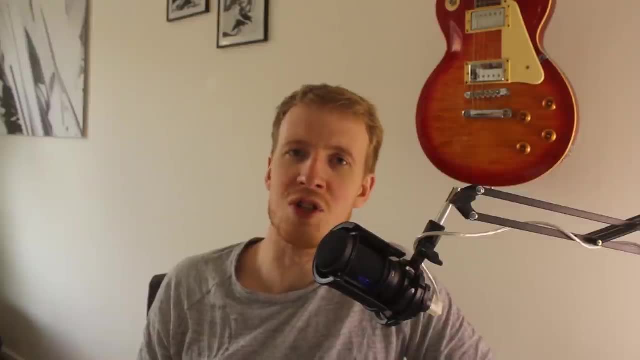 is truly an honor, Anyway. so I'll be talking about the divergence operator here. So this part of the equation of Gauss's law, A normal explanation of this divergence operator is that it kind of measures flow around a vector field. So, for example, if you have a positively 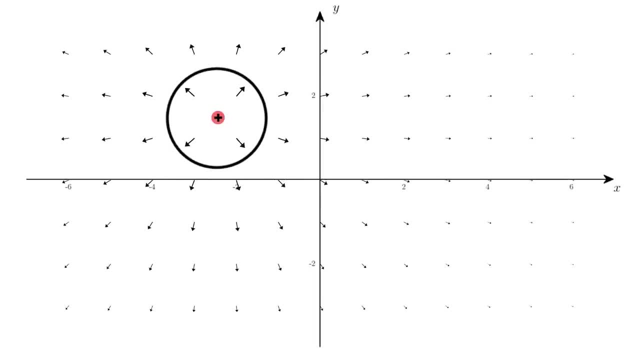 charged particle sitting here. we can see around this circle. here we have an outwards flow of vectors And so we say the divergence is positive. Or in this example, we have a negatively charged particle And around the same region the vectors will point inwards, as if this particle was a sink. 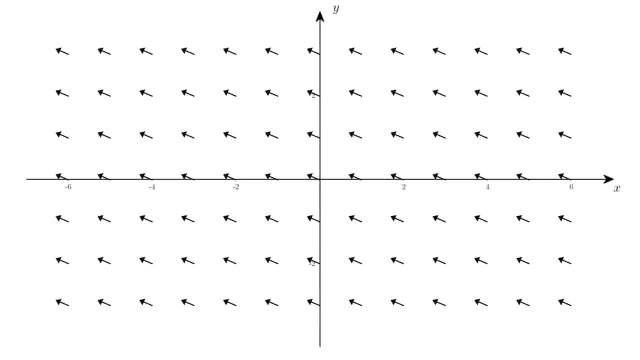 And so we say the divergence around this field here is negative. There's also a different scenario: Vectors just pointing in one direction with the same size. It could be wind moving around with no turbulence, And wherever we put our circle there are as many vectors going in as 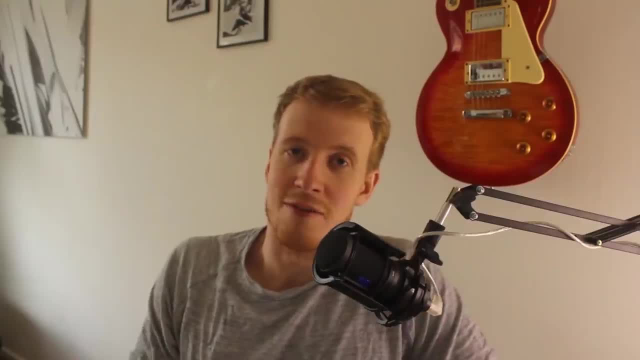 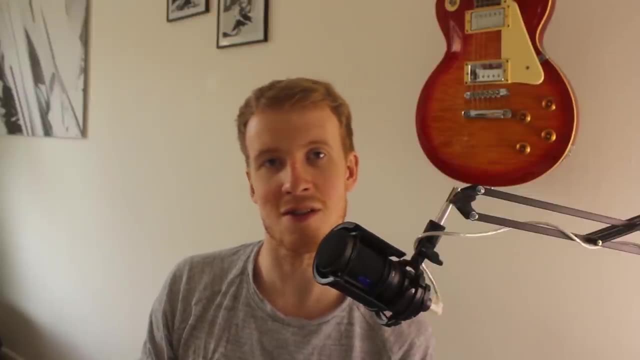 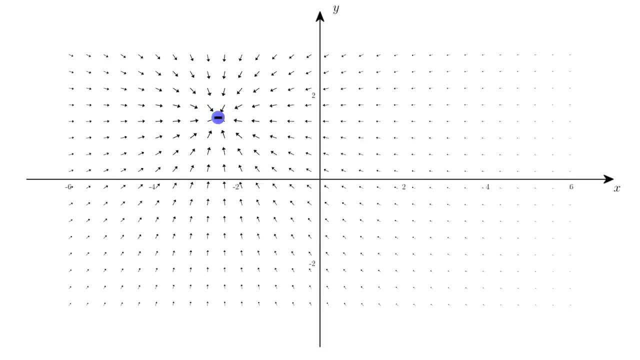 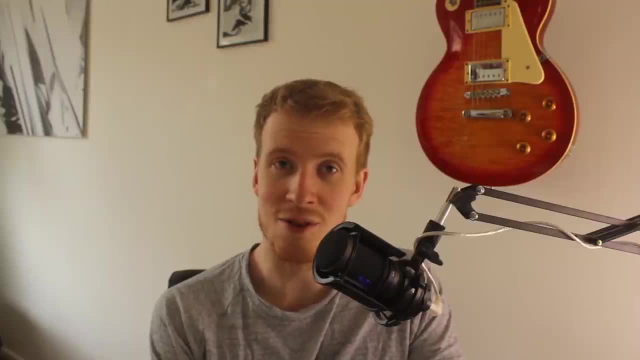 But of course this is just a representation. So in reality there will be infinitely many vectors, just like between one and zero there's infinitely many numbers. And the reason there is an infinite amount of vectors is, of course, because the vector field is given by an equation. So, for example, 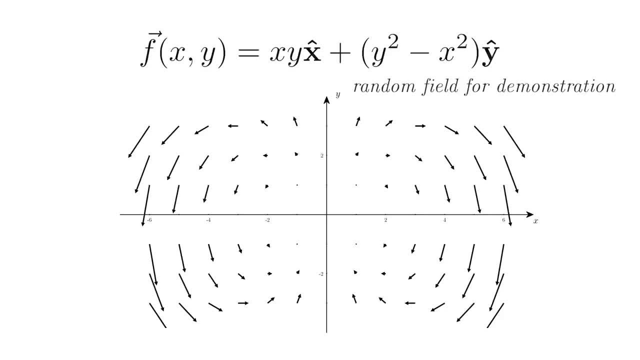 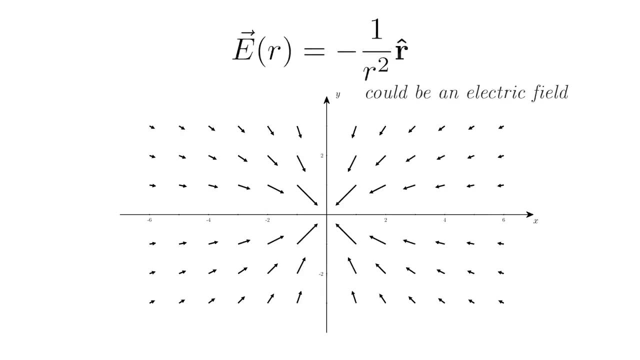 this equation would render this vector field, And again we only draw some vectors. or another equation, one over r squared will result in this field here Now, taking the divergence means that everywhere in this field we measure how much is flowing in or out, Not in the middle, but in the 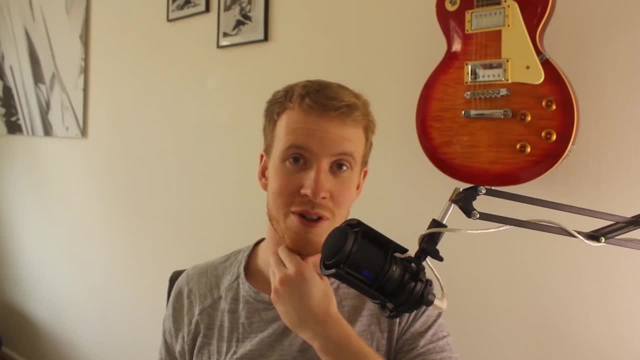 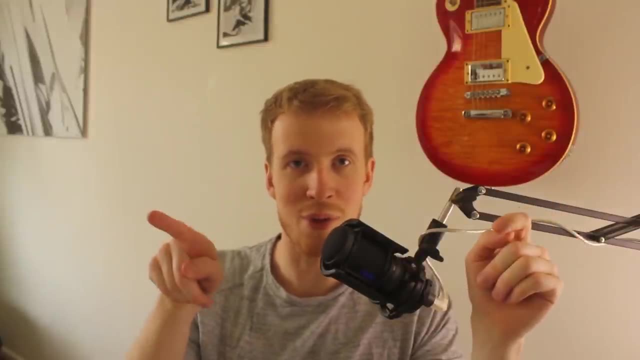 big area but in an infinitely small sphere, or actually point, I guess, And we do that everywhere on the fields. So now, before taking the divergence operator, every point on space had a vector pointing in some direction. But after taking the divergence operator, every point of space has a. 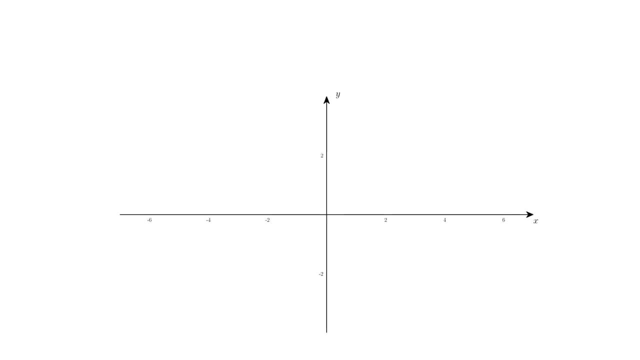 number associated, measuring how much of this vector is flowing in or out. Let's try an example with our previous equations, So let's go back to this one. If we take the divergence of this field, it turns out, if we get this equation, and so when you plug in the numbers, this is what the 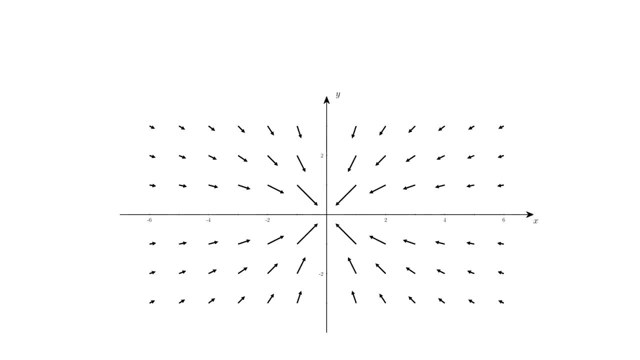 divergence look like. I'll also try with the other example. And here comes something special, because we have a one over r to the power of two. the divergence is zero everywhere. I'm telling you this because that's how charges behaves. So this equation represents an electric field of a charge. 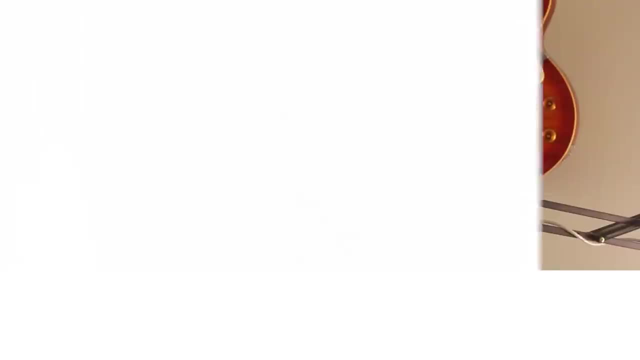 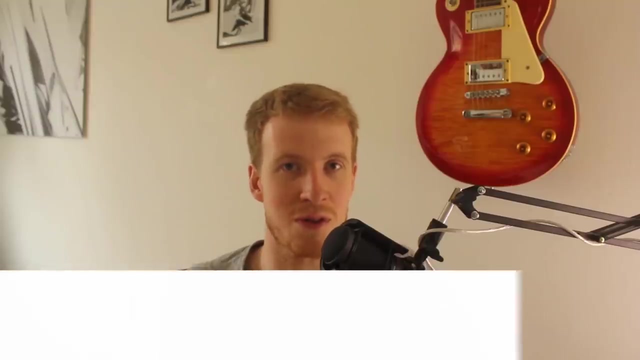 And this is what this equation means. everywhere we don't have a charge, the divergence is zero. So here is zero, here is zero, here is zero. But here we have a charge, And so the divergence equals to the charge density over epsilon zero. I know it might not seem as interesting. 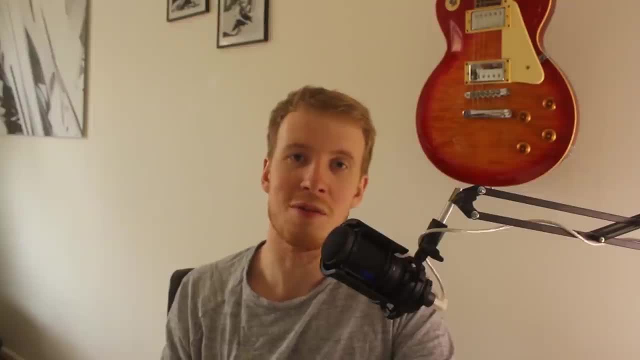 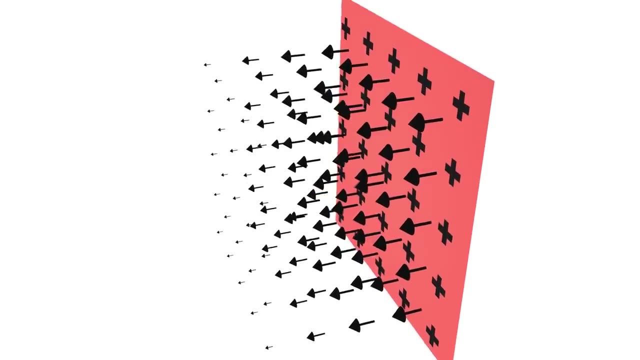 but it's extremely important for calculations where symmetry is special. For example, if you have an infinitely big charge plane- so here we have charges- it will create an E field going out like this. Now we can construct what we call a Gaussian surface. in the E field it's just whatever surface. 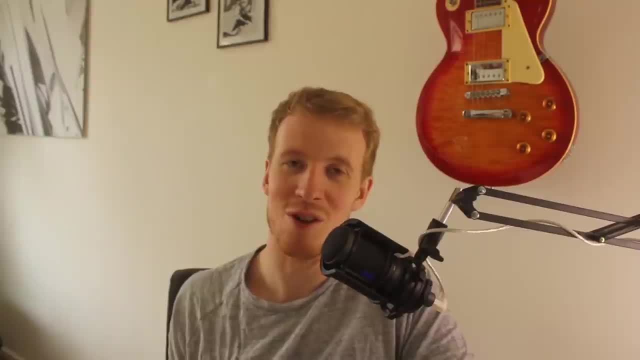 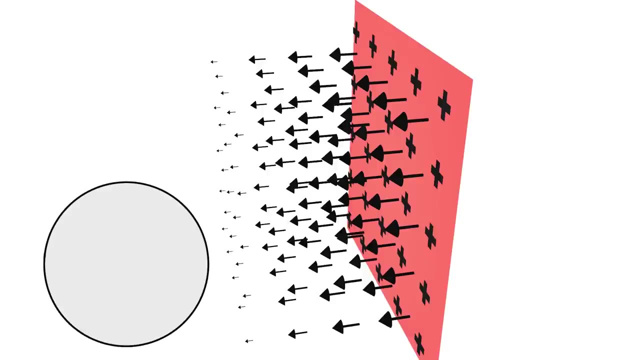 we want, And so the idea is to measure how much is flowing in and out, Because we know the divergence is zero everywhere. we can construct whatever surface we want, So some weird potato, a sphere, a box, or we can construct something that matches the symmetry, such that the calculation will be. 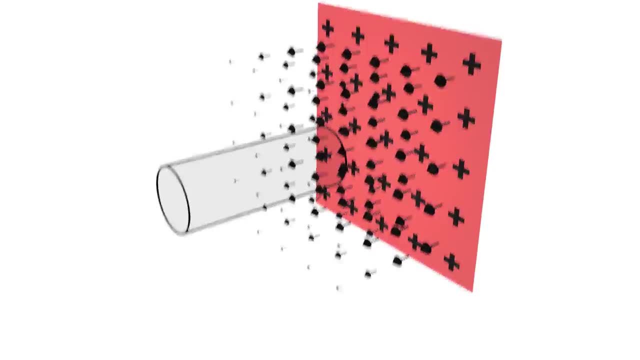 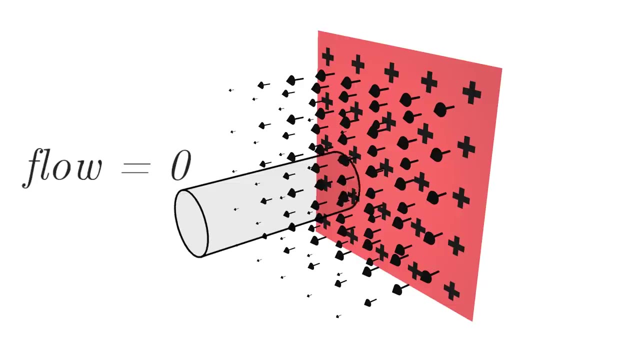 easier to do. So here it is a cylinder. the electric vector field flow will be zero if we don't have any charges in capsules, because the divergence is zero everywhere, And so we can place this Gaussian sphere so it encapsules some of this charge plane, and now we can calculate the electric fields. classic. 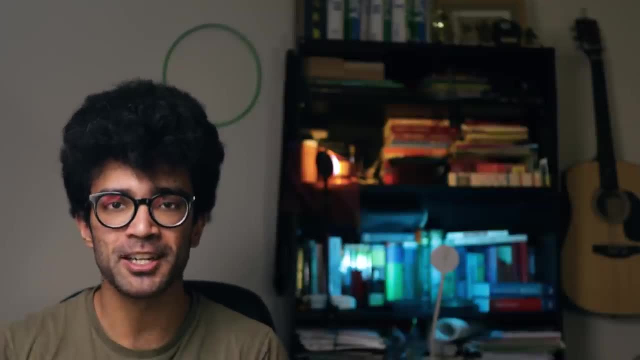 So huge thanks to Mr Higzino for that explanation. If you haven't heard about his YouTube channel or haven't seen any of his videos, then I highly recommend heading over to his channel and giving him a subscribe. As you've seen, he makes some very intuitive and visual videos helping you. 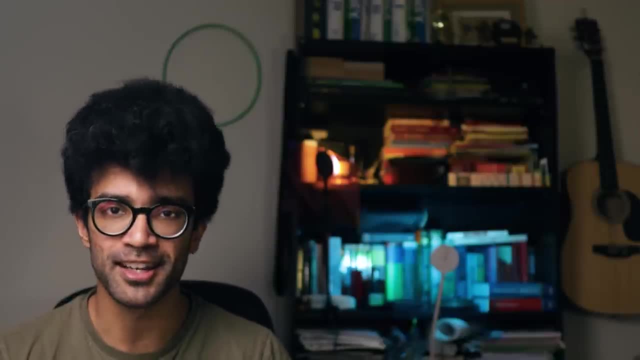 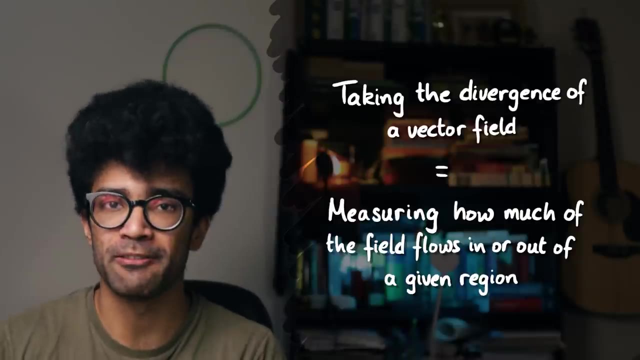 learn different complicated concepts in physics. So head over there and tell him I sent you. But anyway, we've just seen what it means. to take the divergence of a vector field. Essentially we're just measuring how much of that vector field flows in or out of a particular region of space. 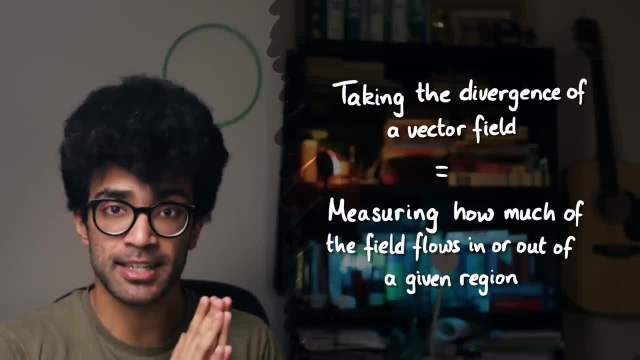 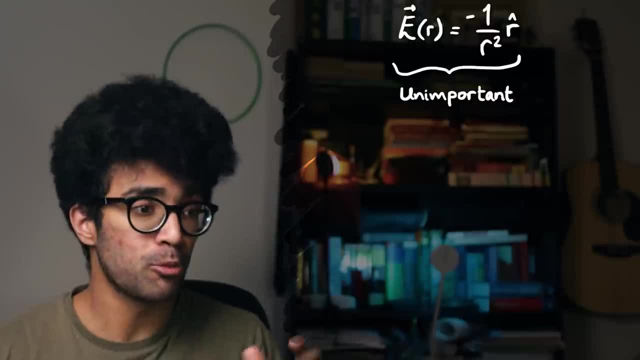 that we happen to be considering. An interesting example we saw in Mr Higz's explanation was the 1 over r squared vector field. Again, we're not too worried about the actual maths of it. We're more worried about what the vector field looks like, what the arrows look like and what direction. 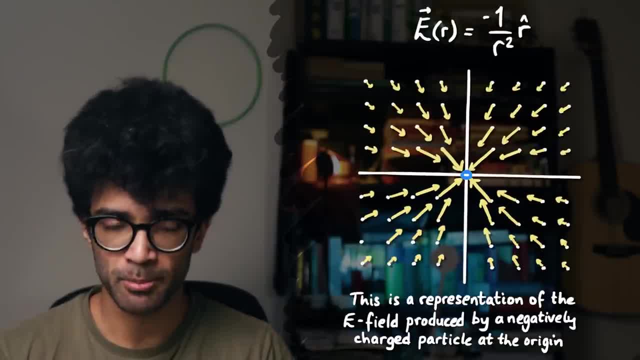 they're pointing in, And so we're going to take the divergence of a vector field and we're going to put it in. Well, as it turns out, a negatively charged particle placed at the origin, in our original vector field, will produce an electric field that looks identical to this. What this? 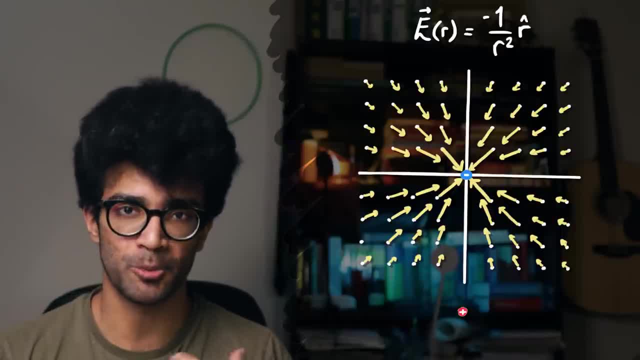 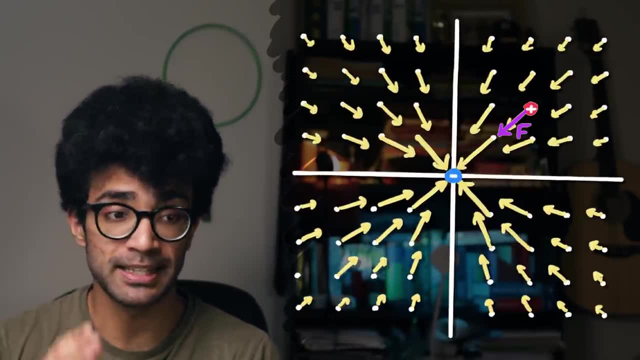 means is we could take another particle, let's say our positively charged particle from earlier, and place it at some point in this electric field. When we do, we see that the force on the positively charged particle in this particular case is pointing toward the. 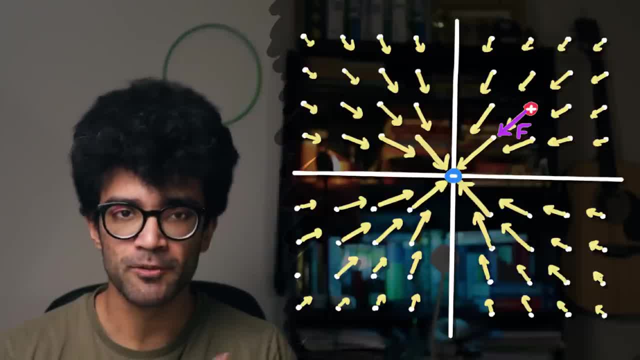 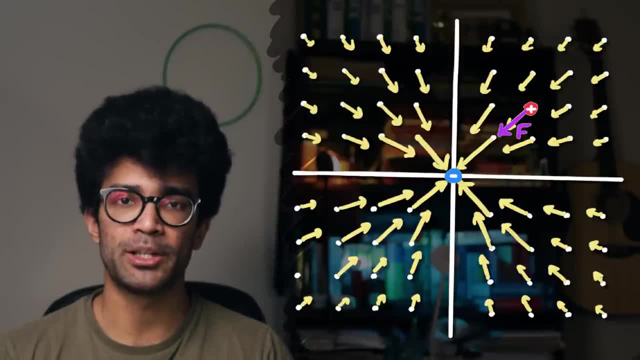 negatively charged particle And this hopefully makes intuitive sense. We've learned, maybe all the way from high school, that positively charged particles and negatively charged particles attract each other. Remember, the convention that we use for electric fields is that the arrows point in the direction of force experienced by a positive 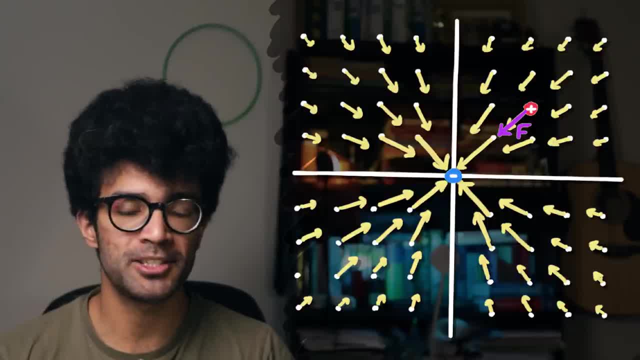 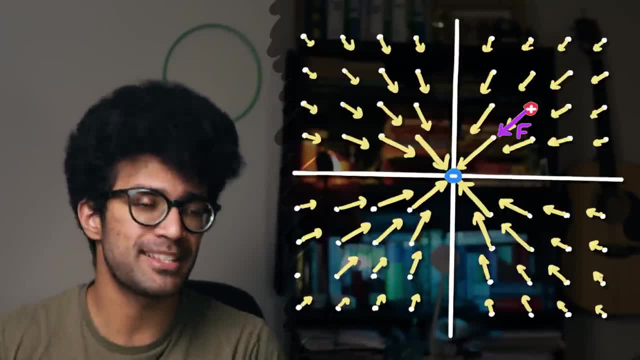 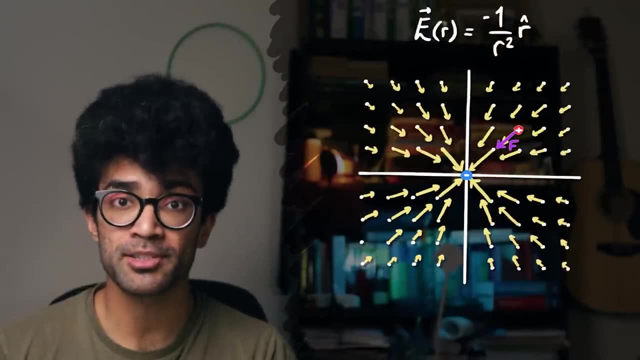 particle placed at that particular point. So we could take our positively charged particle and place it anywhere in this electric field created by the negative particle, And the positive particle would always experience a force pointing toward the negatively charged particle. In other words, they're both attracting each other. And the other interesting thing is that the vectors closer to 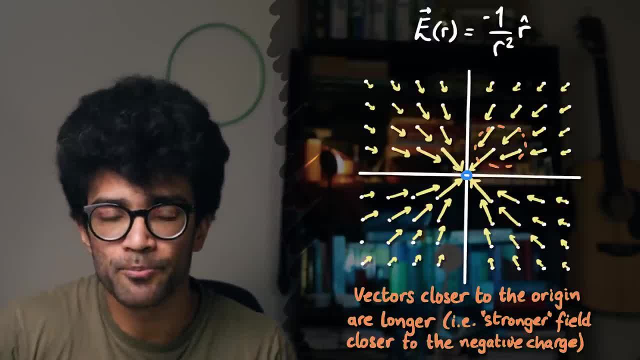 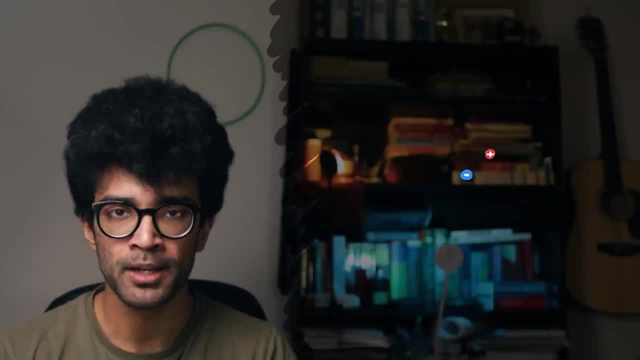 the origin, the charged particle which created the field, are larger, Whereas further away they're smaller, Which also makes intuitive sense in that, let's say, we took a positively charged particle and placed it here. Well, that particle is going to be more strongly attracted to the 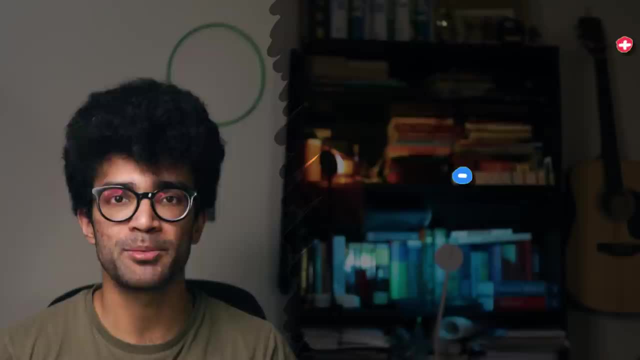 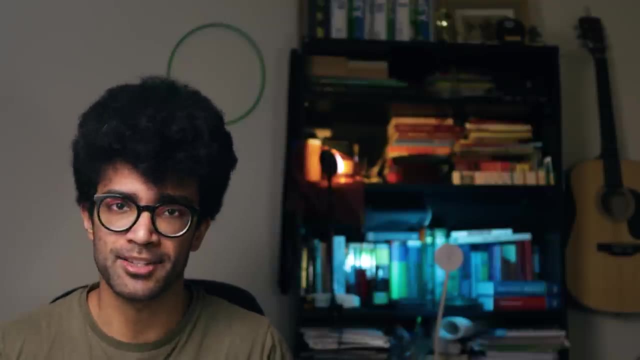 negative particle because it's closer, Whereas if we place it much further away, it's going to be much more weakly attracted to the negatively charged particle. They still attract, they're just much further away, so they don't attract each other as strongly. Let's return to our Maxwell. 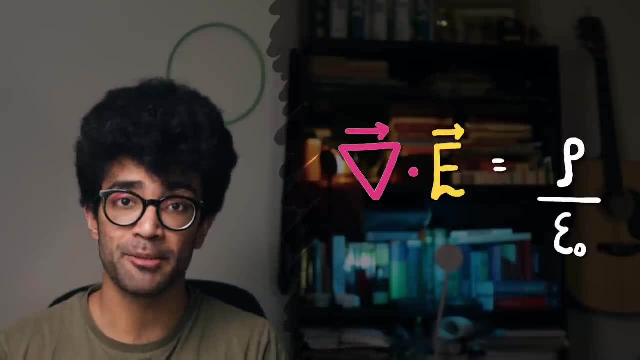 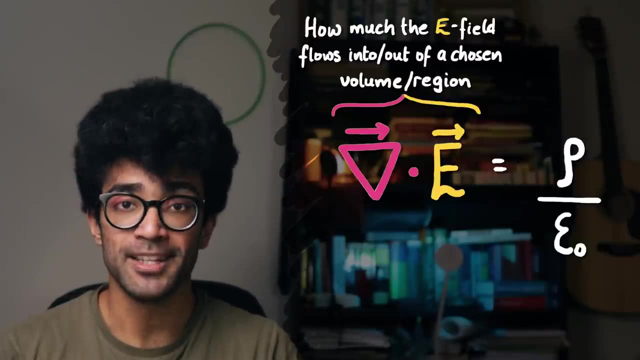 equation. now We've seen that the divergence of our electric field is a measure of how much of that field is flowing in or out of any particular region of space that we want to be considering, And this particular equation is telling us that that divergence is 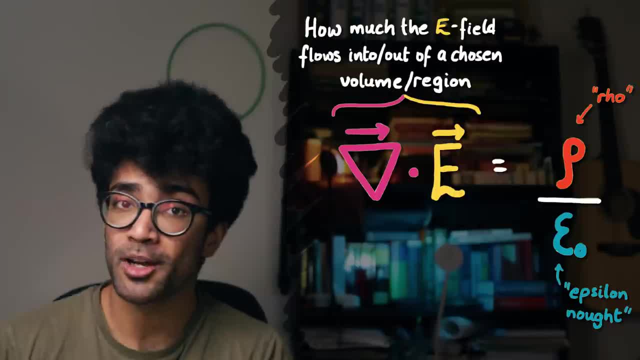 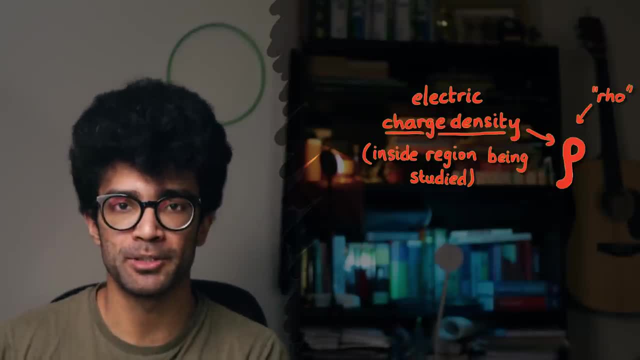 equal to rho divided by epsilon naught. So what are these two quantities, rho and epsilon naught? Well, rho is the electric charge density inside the region of space that we happen to be taking the divergence for. Basically, this means the total charge inside that region divided by the 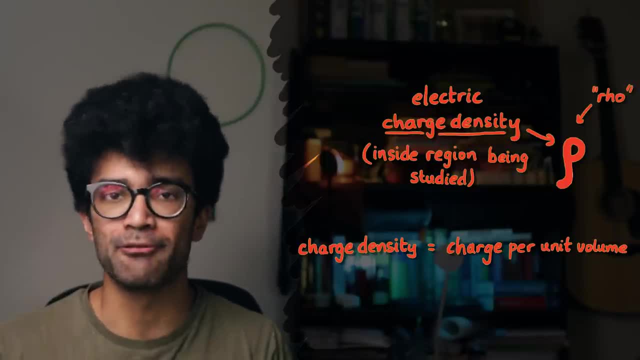 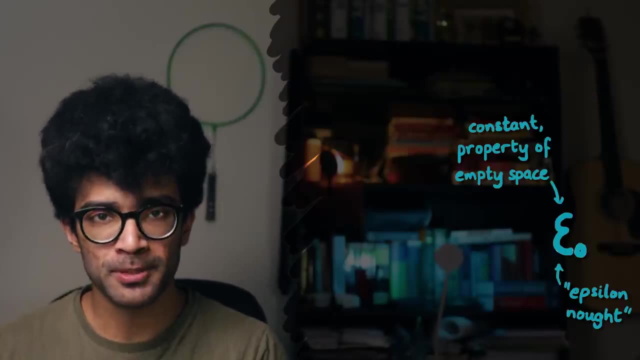 volume of that region. It's the charge per unit volume. We'll look in a bit more detail at this in a second, but let me just quickly explain what epsilon naught is. Epsilon naught is a fundamental property of the vacuum, the empty space of our 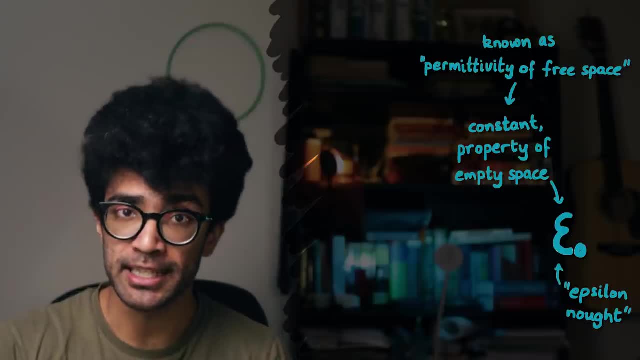 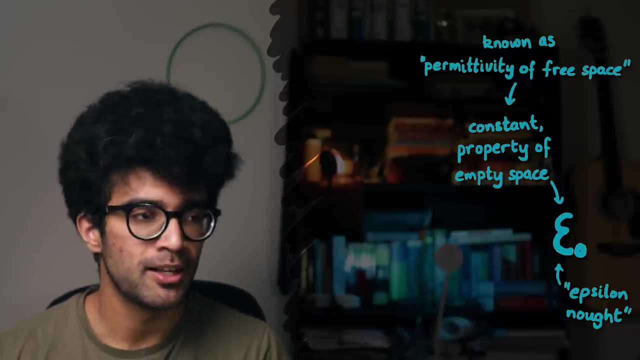 universe. This particular constant of nature is known as the permittivity of free space or vacuum permittivity, And this is a constant that comes up a lot when discussing electromagnetism. I'll talk about this more in a separate video, but for today it just represents a constant. 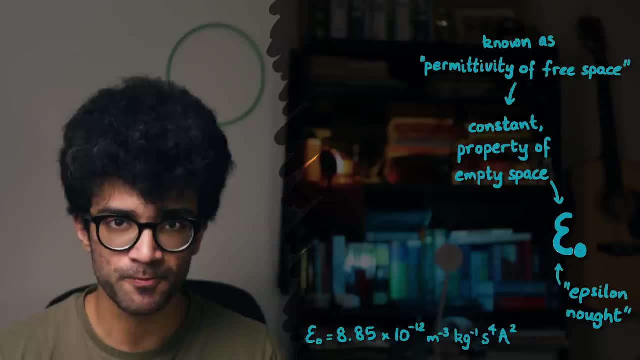 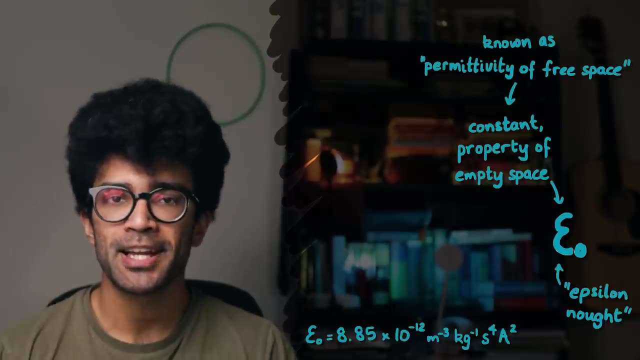 And this constant is a property of vacuum, of empty space, Because what we're securing when we're talking about electric fields is empty space, aside from where we place charges. Let's now look at linking the two sides of our Maxwell equation: the divergence of the 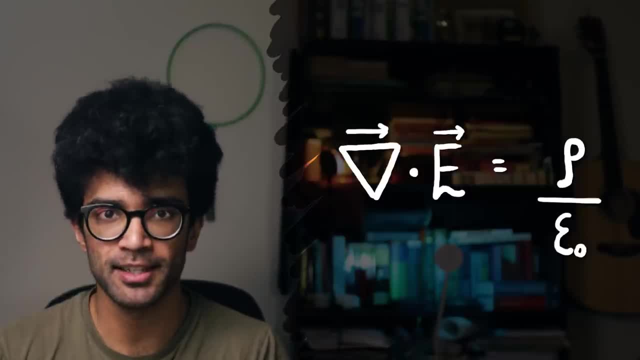 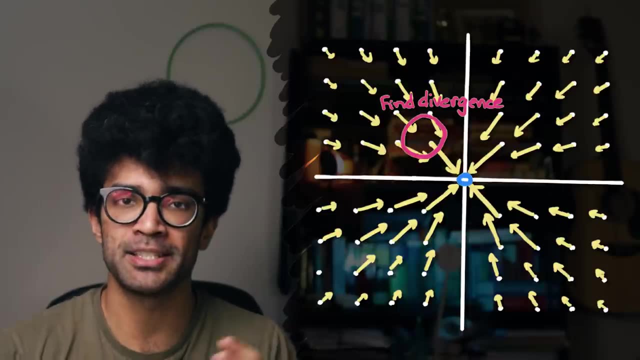 electric field in a particular region of the electric field that we want to consider and the charge density inside that particular region of space. Let's say we want to take the divergence of the electric field in this particular region. here I'm not going to draw 3D, just imagine. 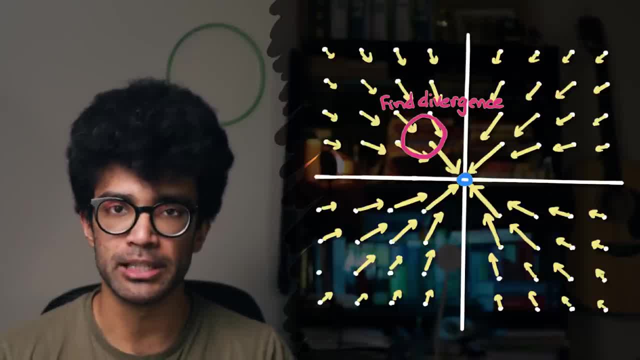 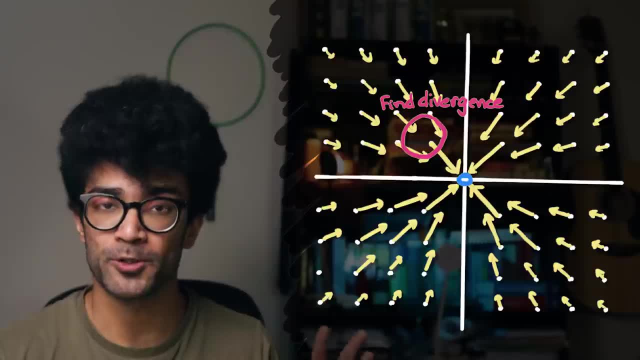 that this is a sphere rather than a circle, And we can see that in this particular region there are vectors pointing into sphere and on the other side there are vectors pointing out, so as much of the vector field flows into our sphere as it does flows out, this means that the flow in is exactly balanced by the flow. 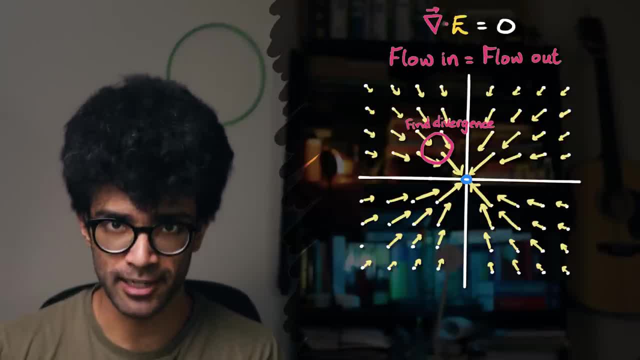 out and the divergence of our electric field in this region is zero, and this exactly works with our maxwell equation, because the charge density in that particular region, for this particular electric field, is zero. there is no charge inside this particular region of space, and so the charge 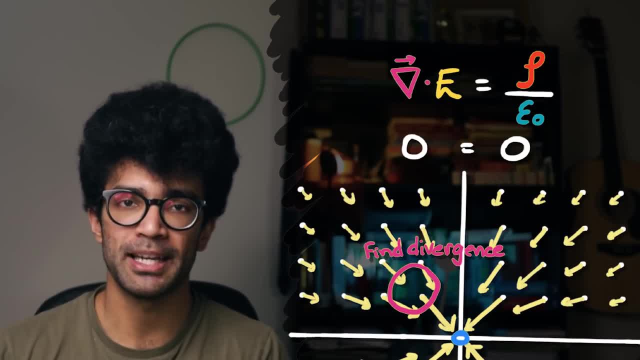 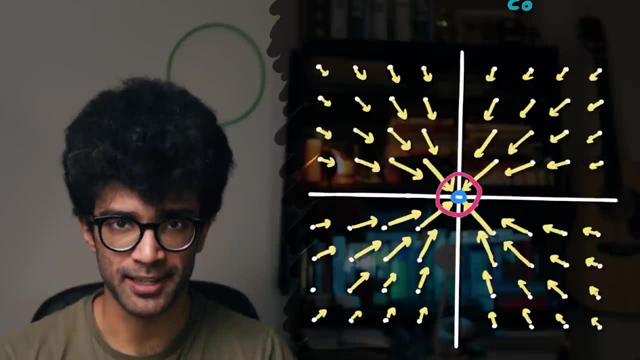 per unit volume is also zero. so for this particular region of space, left hand side is zero, right hand side is zero. equation makes sense. let's now consider this region of space. this gets a bit more interesting. we can see that here all of the vectors are pointing in to the sphere. none are. 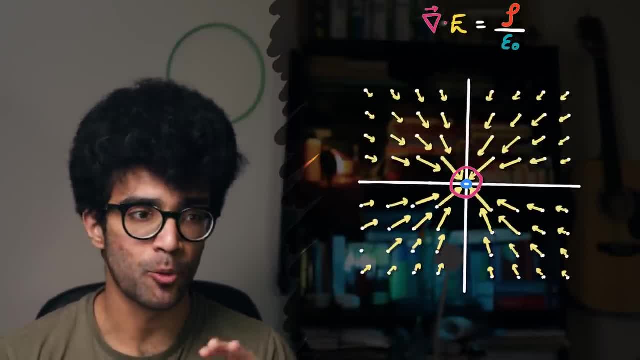 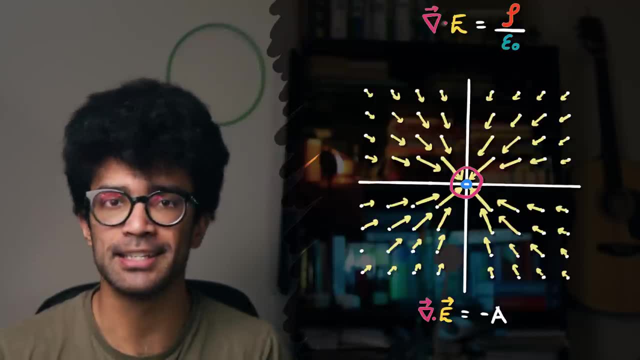 pointing out, and from earlier we said that this conventionally was a negative divergence. so overall, the left hand side of our equation is equal to some negative value. let's call it negative a. it doesn't matter what the exact value is, but the interesting thing is that here it's not. 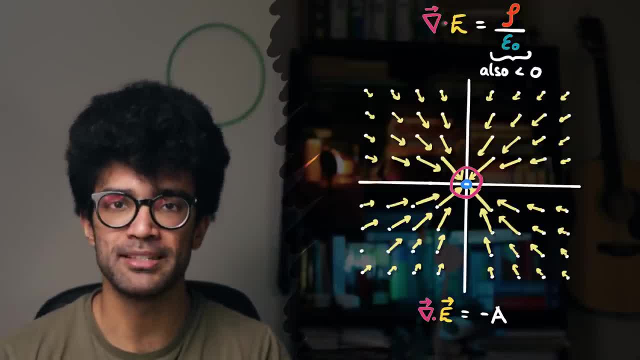 equal to zero, so that's why we don't want to worry about it here, because this equation is not equal to zero, and so this means that the right hand side must also be some negative value, which it is, because, remember, on the right hand side we've got the charge density in that particular region of 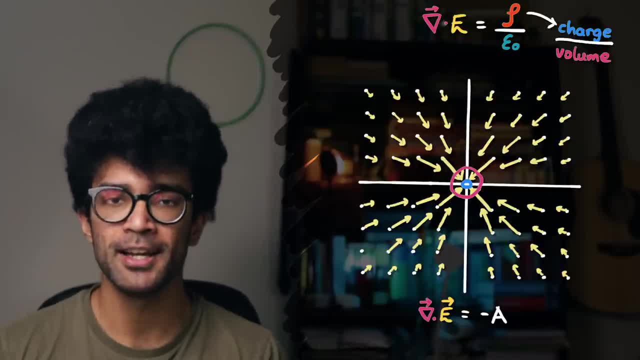 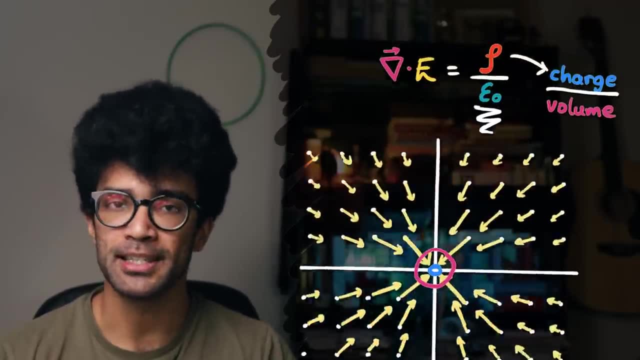 space, which is equal to the charge in that particular region of space divided by the volume of that region. and of course we've got the scaling factor epsilon naught, which, like i said for this video, is just a constant, and so we see that the charge negative q divided by the volume. 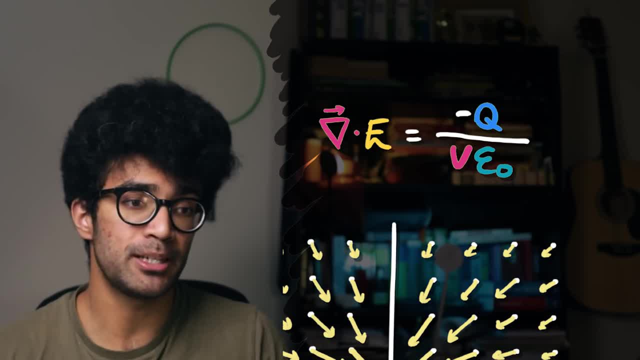 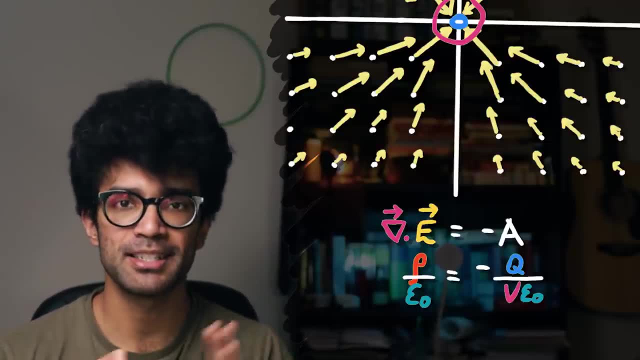 let's call that: v divided by epsilon- naught as well- must be equal to negative a. again, particular values don't matter, but what we see here is that on the left hand side we've got some negative value, and on the right hand side we've got some negative value as well. the equation again makes: 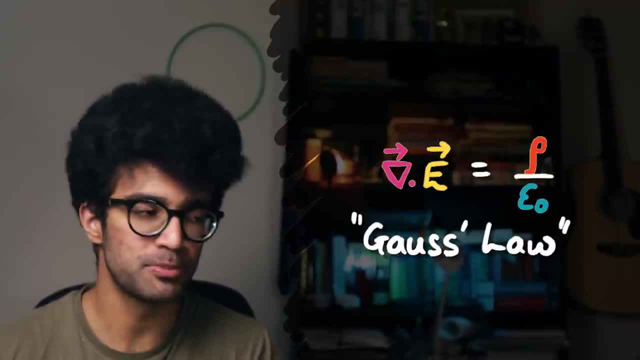 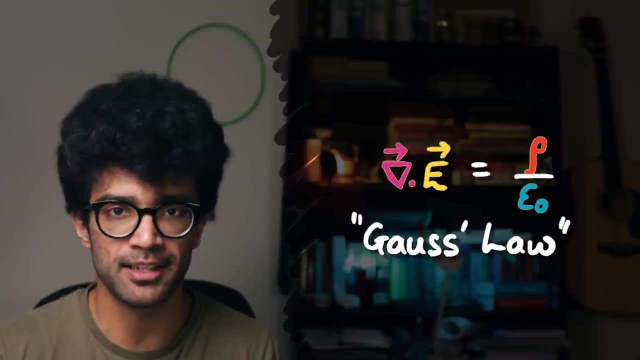 sense. but this equation that we're thinking about- one of maxwell's equations, technically gauss's law, because gauss came up with this first- does a lot more than just mathematically relate the left-hand side of this equation to the right-hand side. in fact it's a prescription as to how electric fields 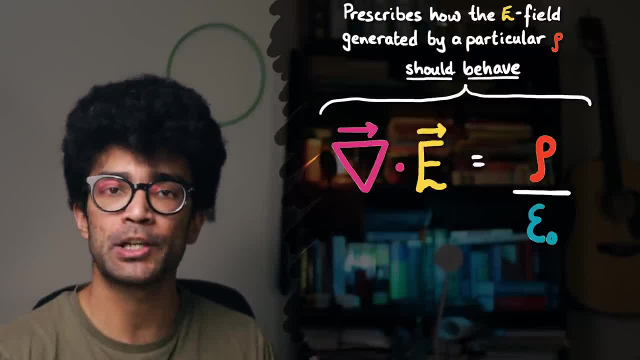 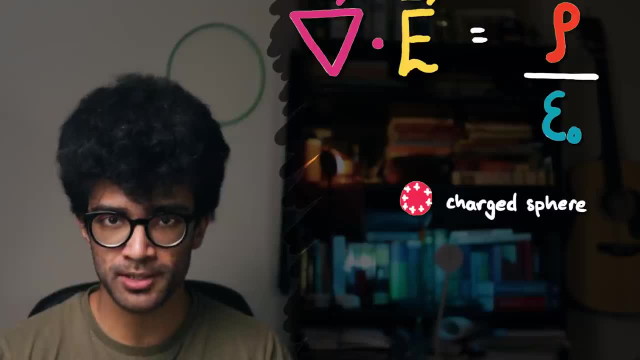 must behave. what this is telling us is that if we have a particular kind of charge, maybe a charged sphere, whether the charge is negative or negative, or positive or negative or negative or negative, or just distributed all over the surface of that sphere, as opposed to just a charged particle, now, 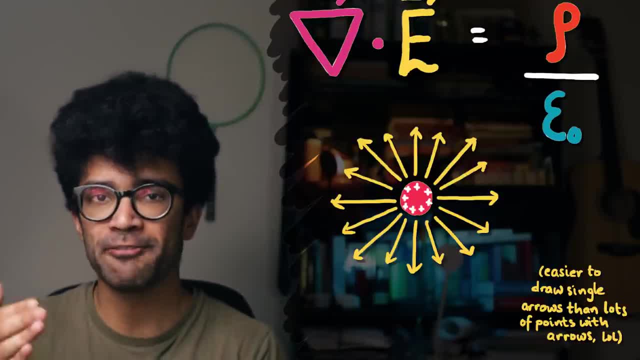 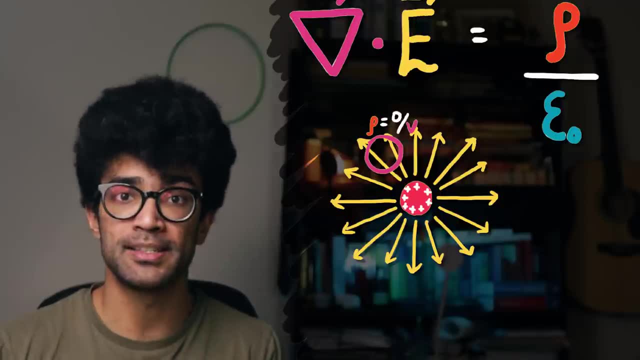 the electric field generated by that charged sphere must behave in a very specific way, and that specific way is the following: the charge density in any volume that we want to consider, any particular volume that we want to consider, divided by epsilon naught, must be equal to the 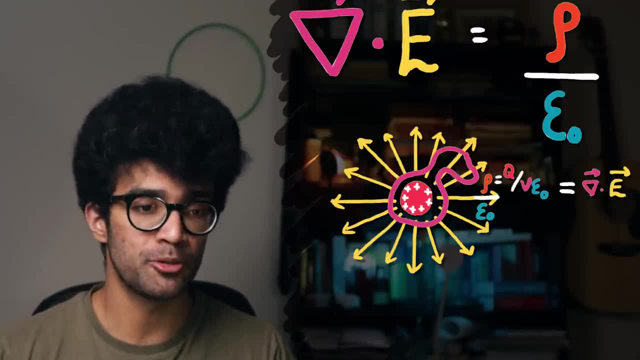 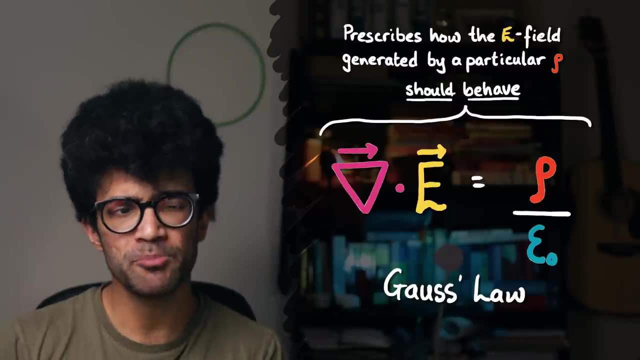 divergence of the electric field. and this isn't just true for a charged sphere or a charged particle, this is true for any distribution of charges. so this particular equation, gauss's law, is very prescriptive. in a way, it tells us the electric field generated has to behave in a very 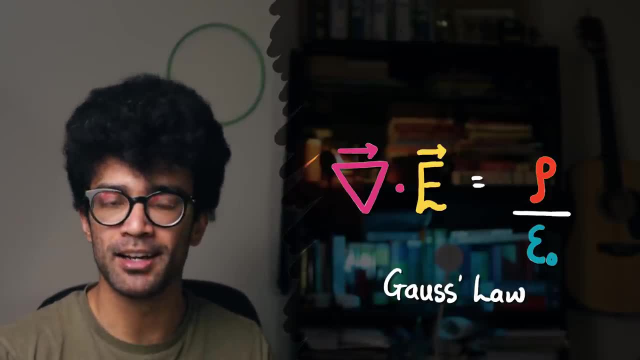 specific way. so that's an overview of this particular equation. here i've simplified many things down and i know that i haven't gone into like the intricacies and the particular details about this equation, but hopefully i've explained it well enough that it makes sense. let me know in. 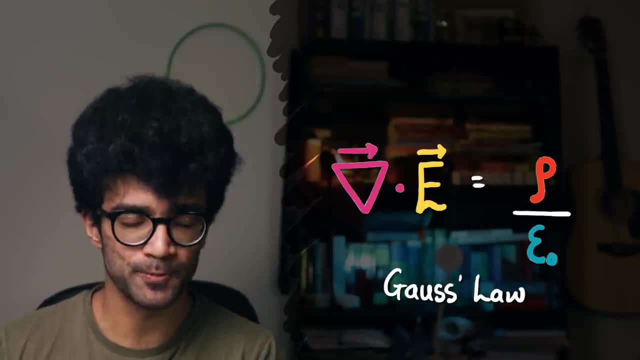 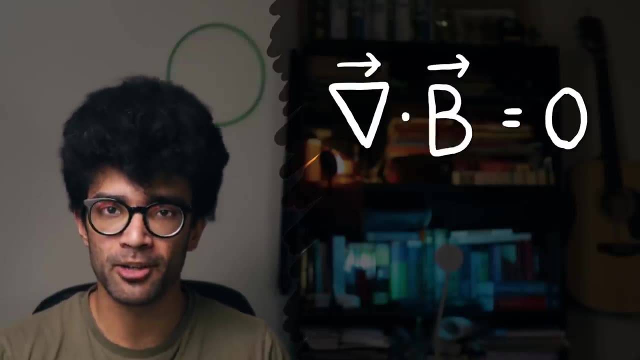 the comments below. if that's not the case, i do have one more thing to talk about, though. i keep talking about the first maxwell equation video that i made a while ago now, and the reason for that is that the equation i talked about in that video is very different from the equation that i 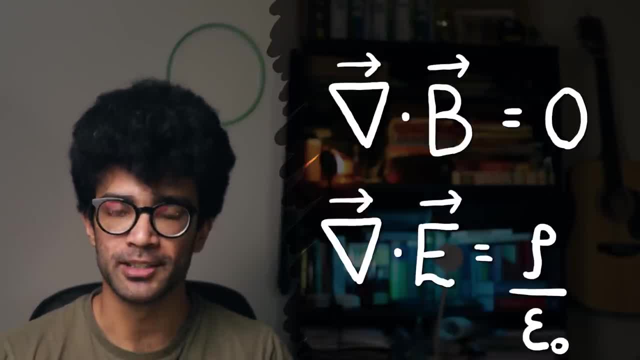 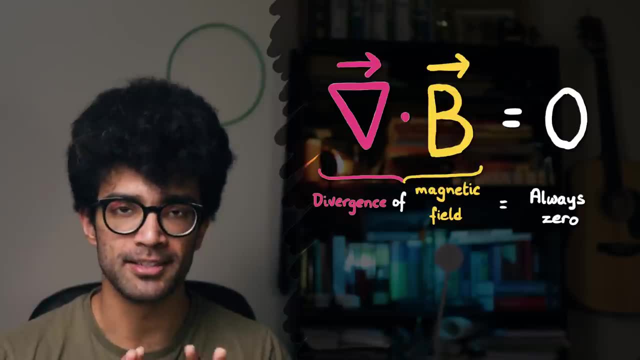 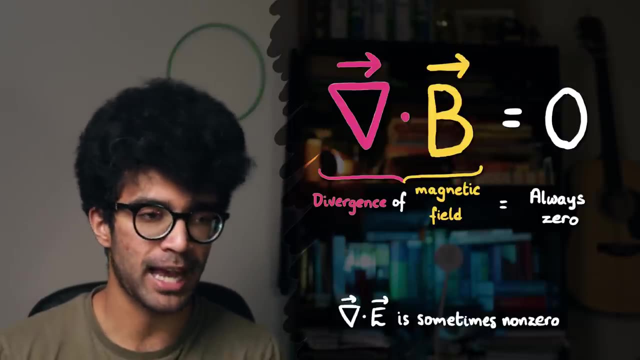 talked about in this video. that equation deals with the divergence of magnetic fields and it tells us that the divergence of magnetic fields is always zero and this shows a fundamental difference between classical electric fields and classical magnetic fields. while electric fields can have a non-zero divergence, they're dependent on the charge density of any particular volume that we